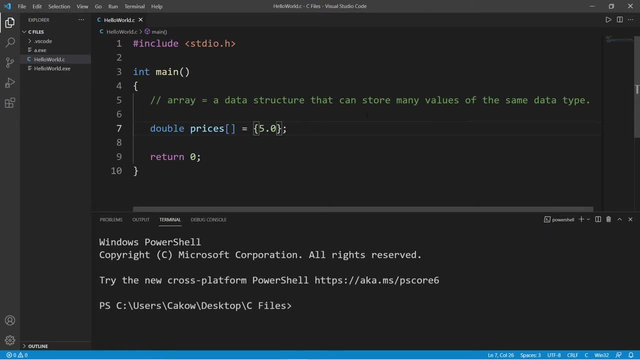 can add multiple values, each separated with a comma. So let's say I have a value of one item in a fictional store of ours and I have the price of $10,, $15,, $25, and maybe $20.. Now you may have noticed some parallels when we 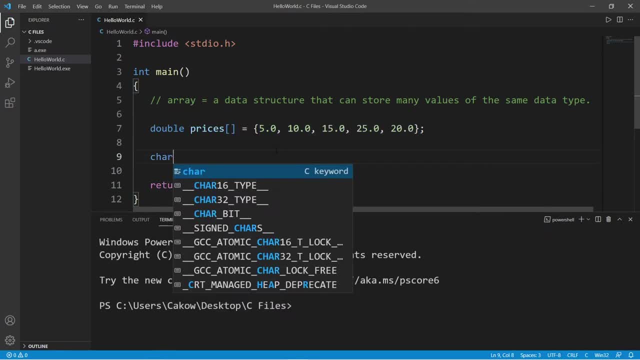 create a string. It's really an array of characters. So if I need a name, we would say the data type is char and we will create a name array followed by a set of square brackets, And I will set this equal to some amount of characters. 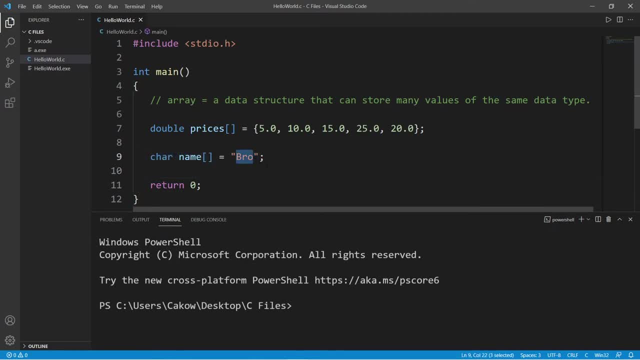 A string is really just an array of individual characters And with my name here I have three individual elements, three individual values. Now, if I need to access one of these values, I need to use an index number. So let's print one of these numbers, So it prints. 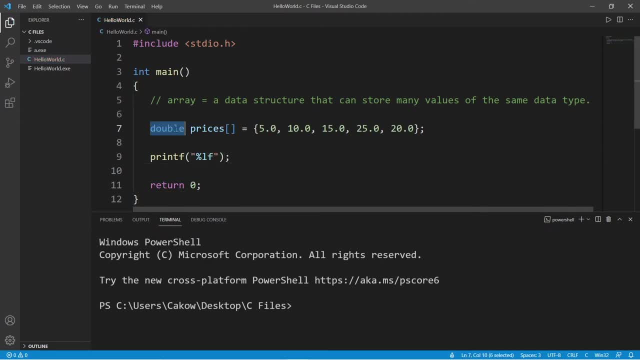 F. I'm going to use the format specifier for a double And I'm going to list my array name- prices- then follow this with a set of straight brackets. then I need an index number So each spot within an array is known as an element. So we have five elements And I'm going to 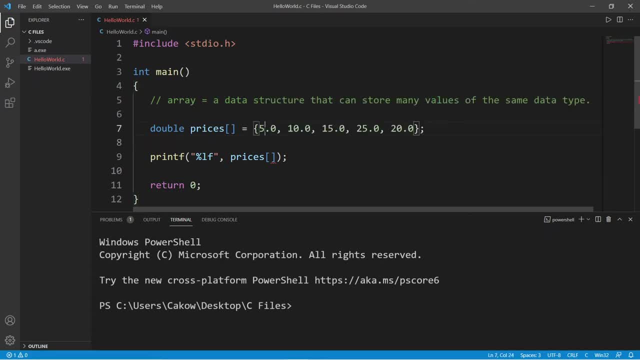 list five elements within our array, And to access one of these elements I need to list an index number. The first element has an index number of zero, because computers always start with zero, So if I display prices at index zero, this contains the number five. 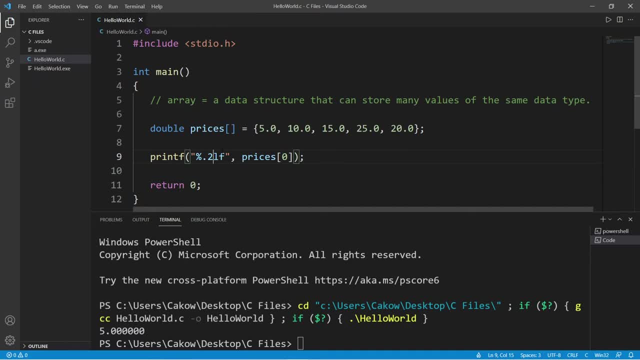 I'm actually going to format this. let's display it two digits after the decimal And I'll precede this number with a dollar sign. Much better, Alright. so then, if I display prices at index two, I'm going to use an index number of $10.. So prices at index two is 15.. Three is 25.. 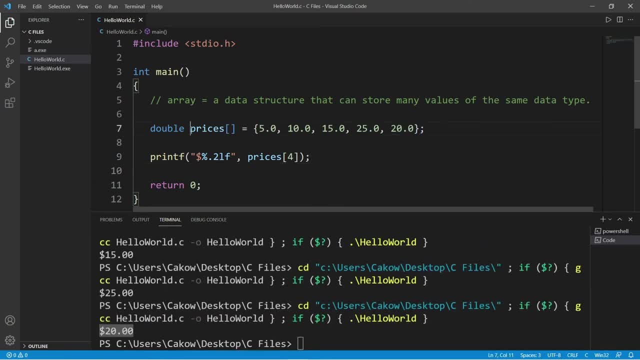 And four, which is our last element, is 20.. So arrays, they have a fixed size. we can't change the size after we compile and run our program. Another thing that you can do too: if you do not know what values you would like to initialize your array with, you can always